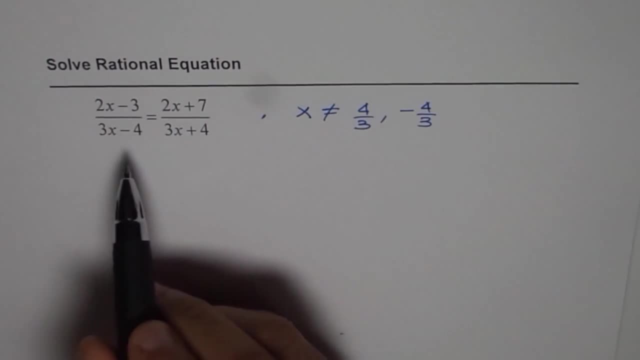 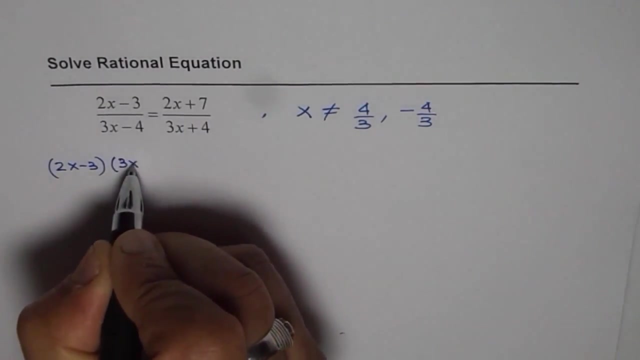 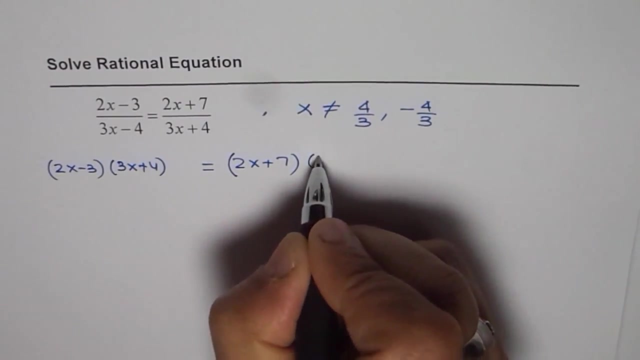 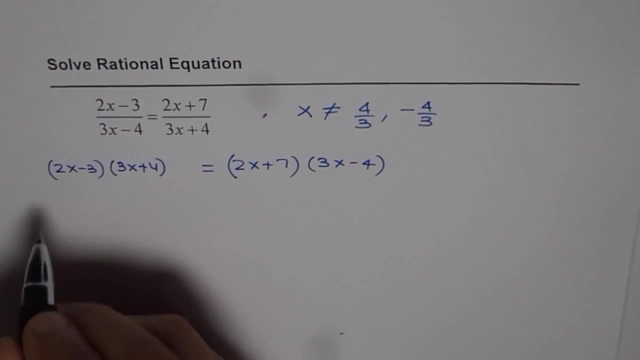 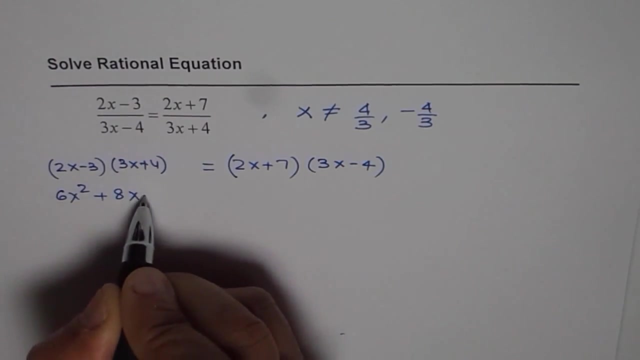 We can cross, multiply and then solve the equation. So that means we get 2x minus 3 times 3x plus 4 equals to 2x plus 7 times 3x minus 4.. Now we can apply the distributive property and expand. 2x times 3x is 6x squared. 2x plus 4 times 4 is 8x minus 9x. 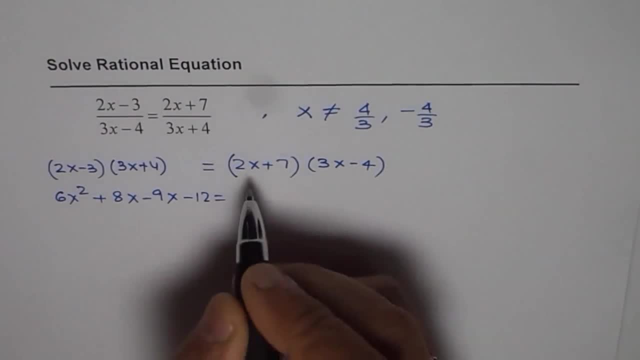 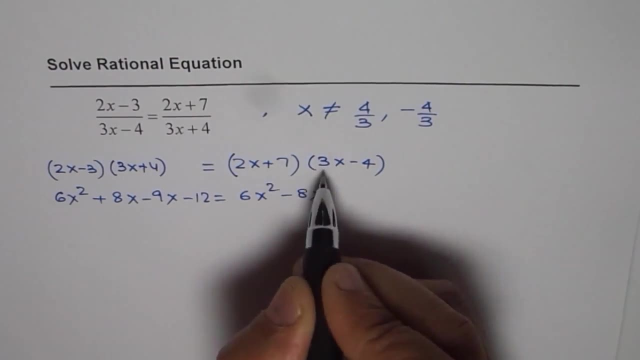 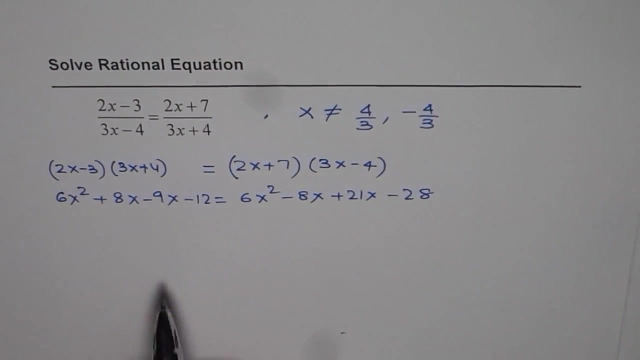 And minus 12 equals to 2 times 3, is 6x squared. 2 times 4 minus 9 is 8x. 7 times 3 is 21.. 7 times 4 minus 28.. So we are having a quadratic equation: 6x squared. 6x squared will cancel. 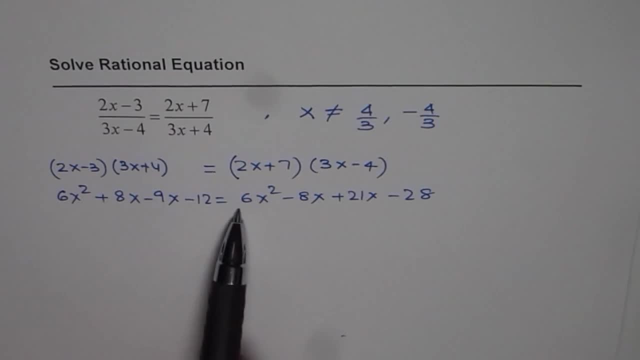 8x plus 9x, So we can bring all these x terms together, The variable terms And constants, to the right side in this particular case. So we and simplify right. So what we have here is: So we can cancel out 6x squared and 6x squared right. So that simplifies. 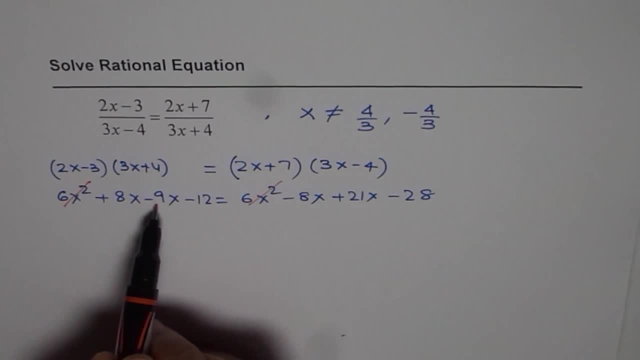 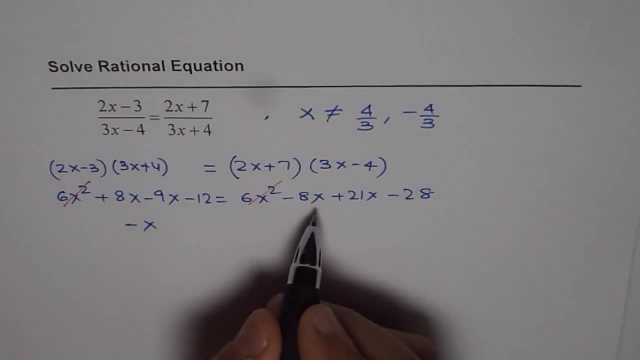 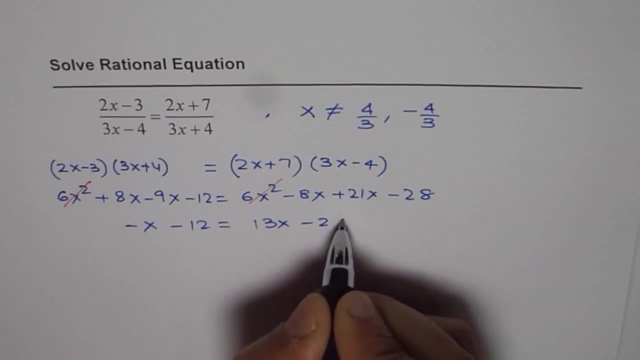 And we have here 8x minus 9x, which is which is minus x. We let's write: minus x minus 12 equals. minus x minus 12 equals 2.. Minus 8 plus 21 will give us 13x minus 28.. 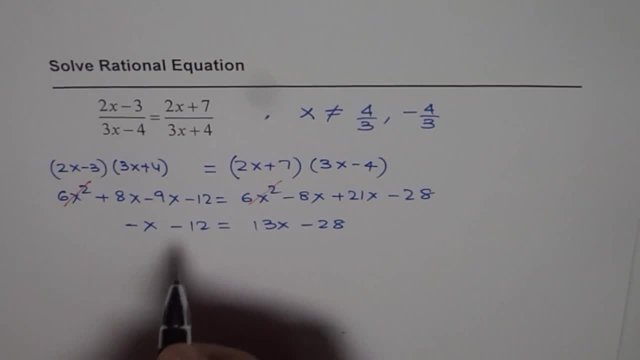 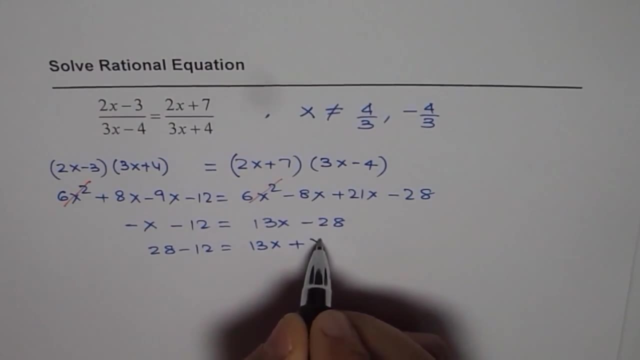 So let's bring x on one side and the numbers on the other side, So we get 28 minus 12 equals to 13x plus x. So we get 14x equals 2.. When you take away, you get 6.. 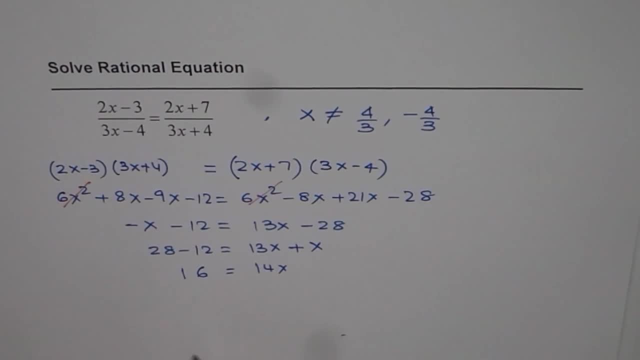 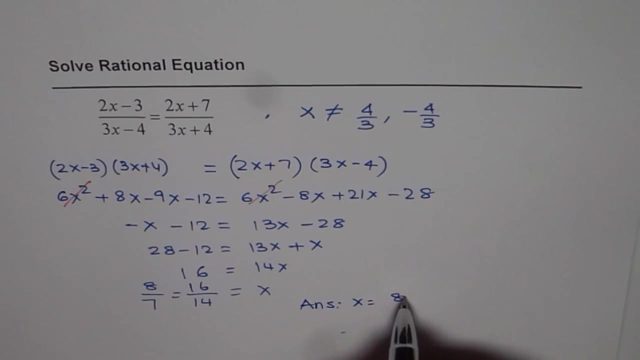 And you get 16 here, right. So we can divide by 14 and get the value of x as 16 over 14. Which simplifies to 8 over 7.. So we have solution here and the answer is: x equals to 8 over 7.. 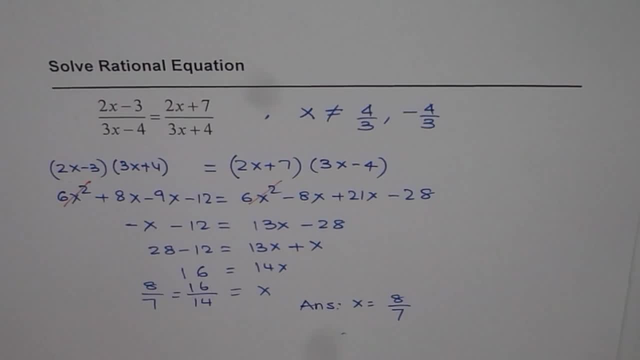 Of course, those are the restrictions, And remember we should check whether the answer is one of these restrictions or not. In this case it is not. So this is our answer, Thank you.